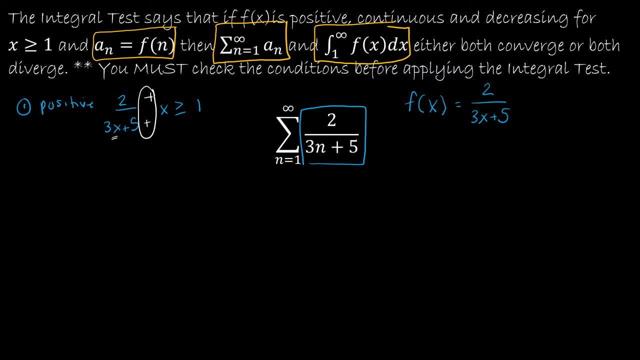 and see if I can get the answer. So f of x is greater than or equal to 1, and if I have a positive over a positive, then my result is positive. So f of x is greater than 0 or positive. So that condition is met. Is it continuous? Well, if I think about, 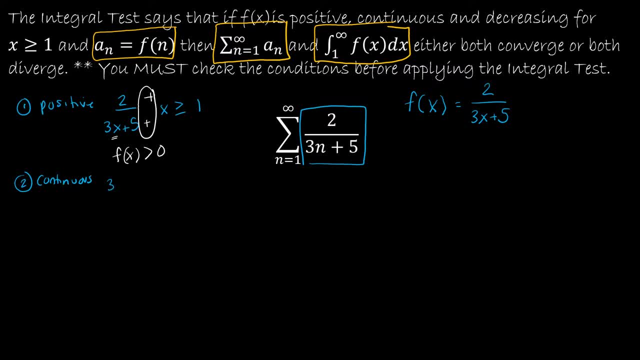 where a rational function is discontinuous. I know that 3x plus 5 cannot be 0. So 3x cannot be negative 5.. So x cannot be negative 5 thirds. but we already know that x is going to be greater than or equal to 1, and so therefore it's continuous. So continuous for x is greater. 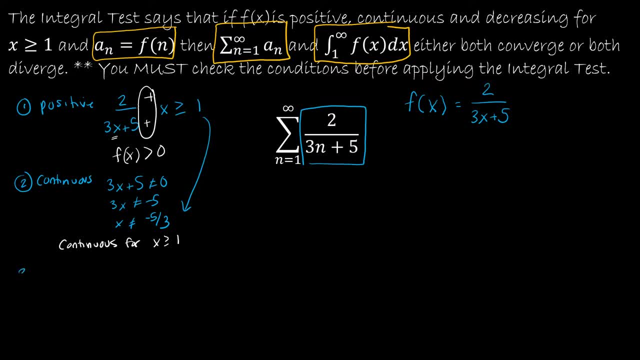 than or equal to 1.. So far, so good. The last one is that I have to show that it's decreasing And to show that it's decreasing again. the easiest way to do that is to show that it's decreasing. The easiest way is to find the derivative of the function. So if I take f, 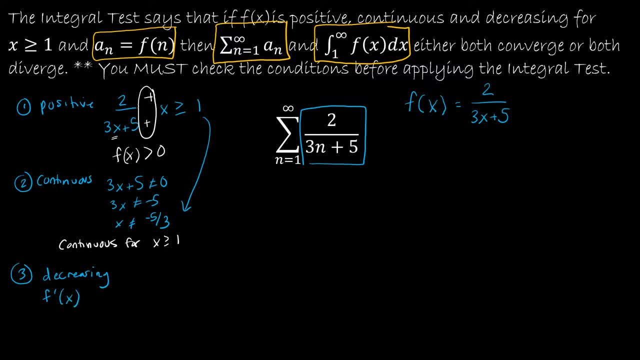 prime of x, and remember f of x- is 2 over 3x minus 5, or 2 times 3x plus 5 to the negative. first, Using the power rule, the derivative of that is negative 2 times 3x plus 5 to the. 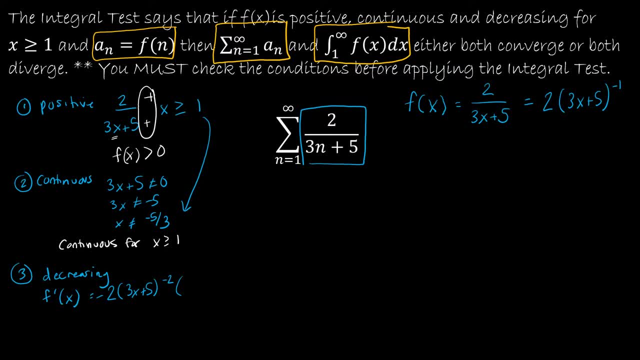 negative 2 times the derivative of 3x plus 5, which is 3.. So f prime of x is negative 6 over 3x plus 5, squared. Doing the exact same thing I did on my first condition. the guy on top is always negative because it's negative 6.. 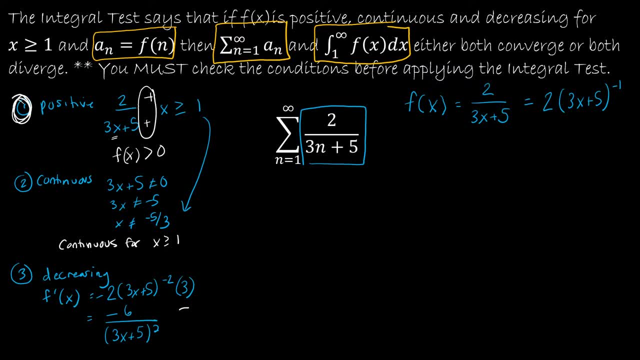 The guy on the bottom, 3x plus 5, quantity squared is always positive And if I take a negative divided by a positive, that value is always negative. So this is less than 0. And therefore this is decreasing Since f prime of x is less than 0.. So I have to check all of 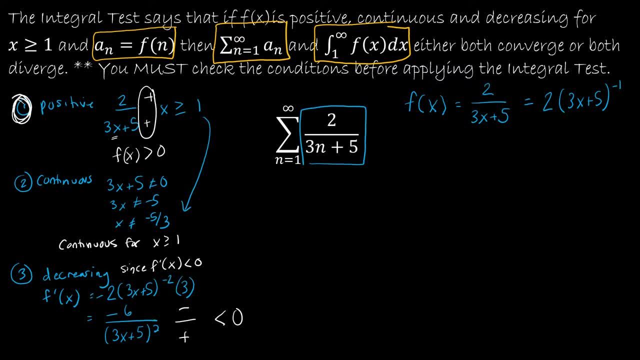 those conditions. And then I say: since f of x is positive, continuous and decreasing, I can use the integral Test. Now, what does the integral test say? The integral test says that both of these guys are going to have the same convergence. 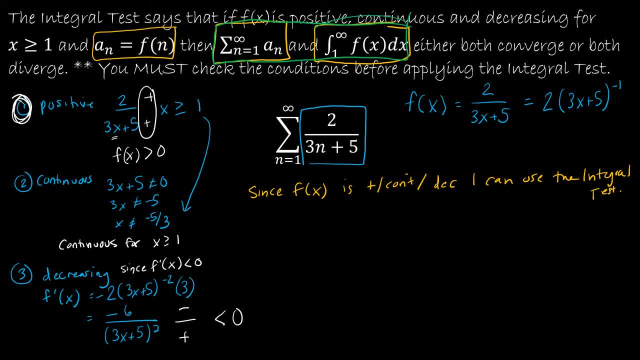 or divergence. So that means I'm going to use the integral from 1 to infinity of f, of x or 2 over 3x plus 5 dx, And I'm going to determine if that converges or diverges. So let's go with it. u is going to be 3x plus 5, so du is. 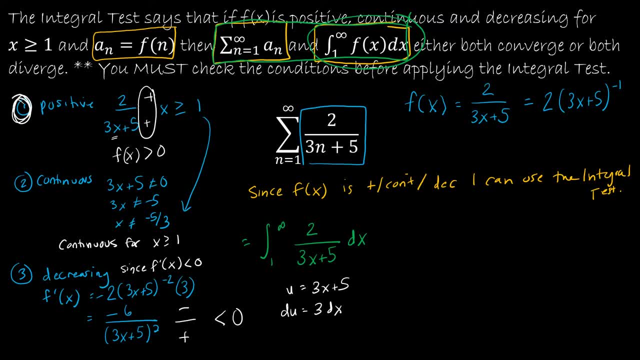 going to be 3dx, So I can think about this integral as again moving this 2 to the outside, keeping in mind that I'm going to need a 3 up here. I'm going to have a one-third out here, So I have. 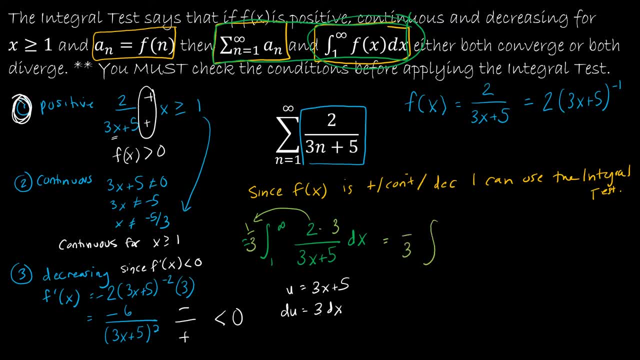 one-third times the integral, I'm sorry, two-thirds times the integral of 3dx over 3x plus 5, and therefore my result is two-thirds. And then, remember, this is just u to the negative 1, and therefore my integral is the natural log of the absolute value of u. 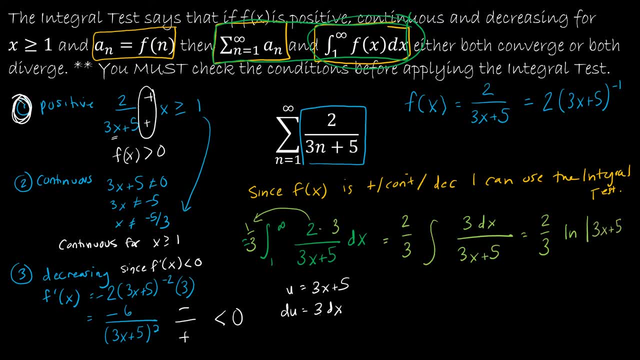 or the absolute value of u. So the natural log of 3x plus 5 from 1 to infinity. So from 1 to infinity. again I'm going to take infinity. I've got two-thirds natural log of what is essentially infinity minus two-thirds times the. 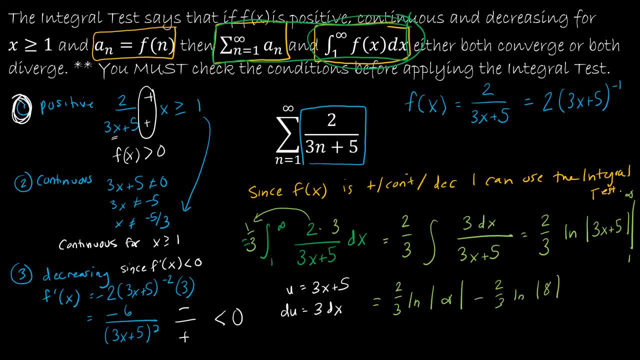 natural log of 8.. Now, two-thirds times the natural log of 8 doesn't mean anything in terms of the big scheme of things, Because I need to think about what does the natural log function look like? And it looks something like this: And as x approaches infinity, the natural log approaches infinity. So this: 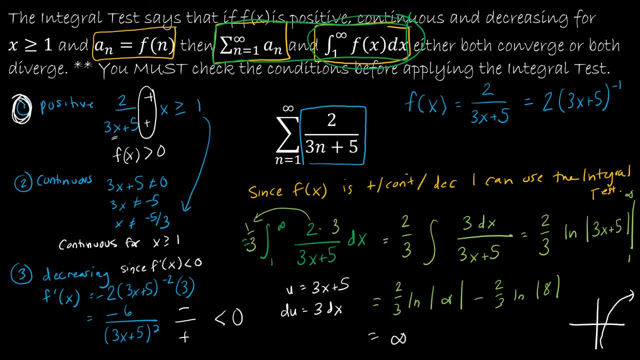 is infinity. What does that mean? That means that the integral diverges and I don't have enough room to write the sentence I would normally write- but you should have plenty of room to write- and says: because the integral diverges using the integral test, And of course, you would have all of this. 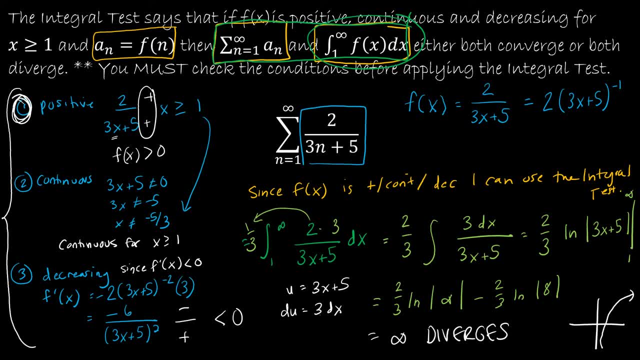 stuff to show me that the integral test is okay to use. But because the integral diverges using the integral test, then the summation diverges. Now one thing I want to point out before we move forward is if you get that the integral converges, the integral test will not tell you what it. 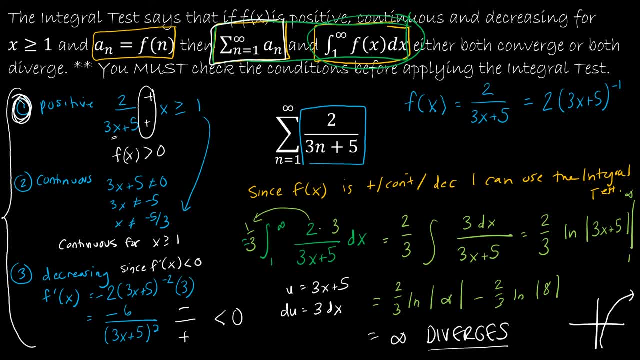 converges to. So it's only going to tell you what it converges to. So it's only going to tell you what it converges to, And that is going to tell us whether it converges or diverges, but it's not going to tell us the value. 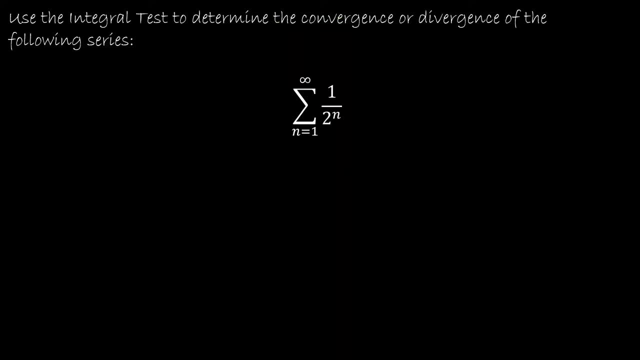 to which the integral converges to. Let's take a look at another example. We were to use the integral test to determine the conversions or divergence of the series. The summation is: n goes from 1 to infinity, of 1 over 2 to the n. So again we need to check one. is this positive? So 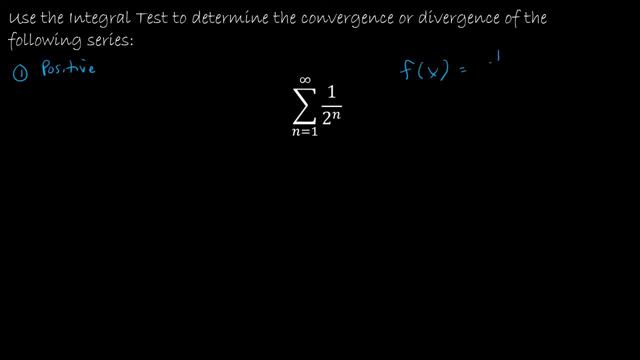 we're going to think of f, of x, 1 over 2 to the x. So is that a positive function? Well, remember that x is going to go be greater than or equal to 1, essentially So 1 over 2, and 1 over 2, squared is 1 over 4,. 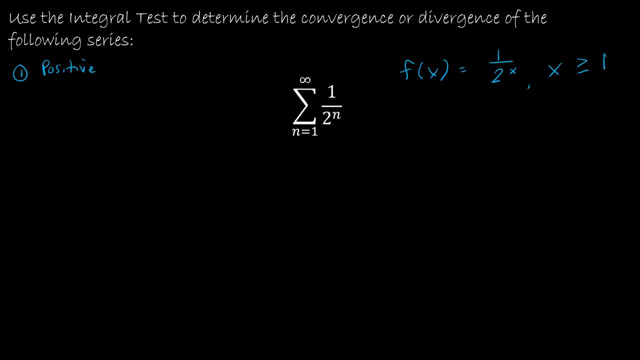 and 1 over 2 to the third is 1 over 8. And so this is positive for sure. So f of x is greater than 0.. 2, is this continuous? Well, the only time that it's not going to be continuous is if 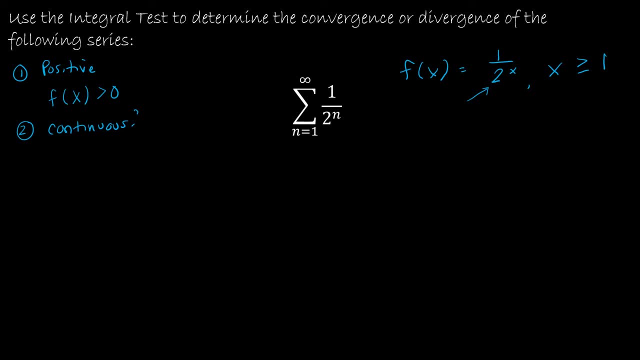 2 to the x was equal to 0, which is not going to happen where x is greater than or equal to 1.. So again, f of x is continuous For 3,. 3 is decreasing And we already saw that. 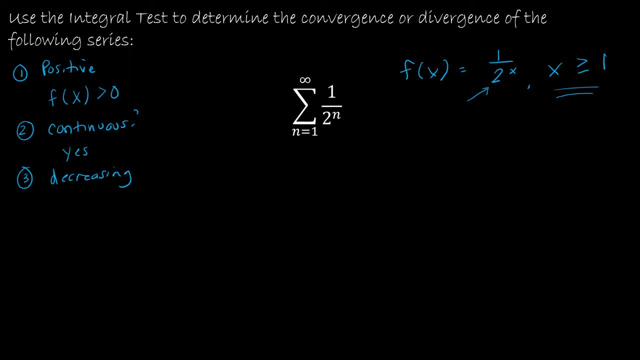 sort of took a look at some of the initial values, but we should take a look at f prime of x. f prime of x, for f of x is equal to essentially 2 to the negative. x would be negative natural log of 2, 2 to the negative x And if I'm looking at that for values where x is greater than or equal to 1,. 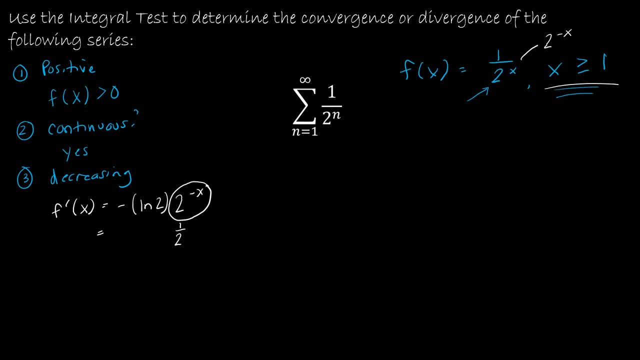 remember, 2 to the negative, x is just 1 over 2 to the x And so this value is going to be positive. Natural log positive negative says I have a negative times, a positive times, a positive. That result is negative. So f prime of x is always going to be less than 0.. 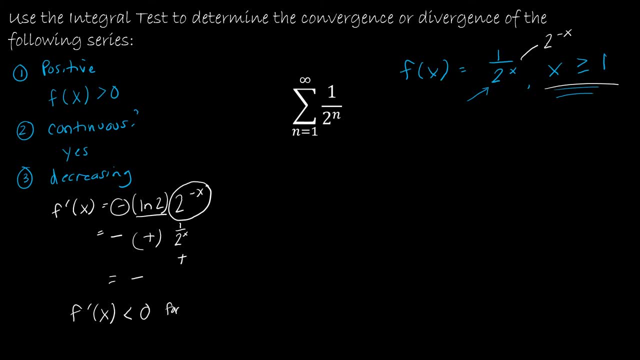 It's always going to be negative, for x is greater than or equal to 1.. So because all of those conditions are met, I can use the integral test. So since all conditions met, I can use the integral test. So rest 70 to infinity 2x with f. 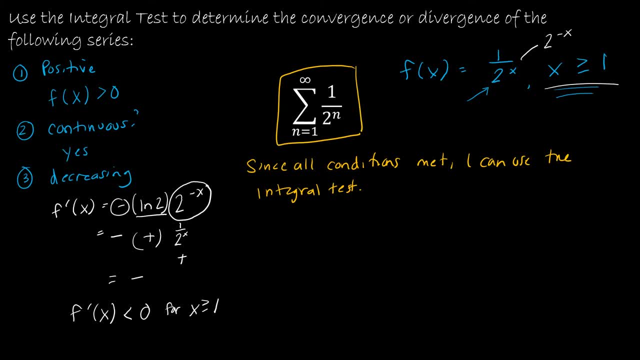 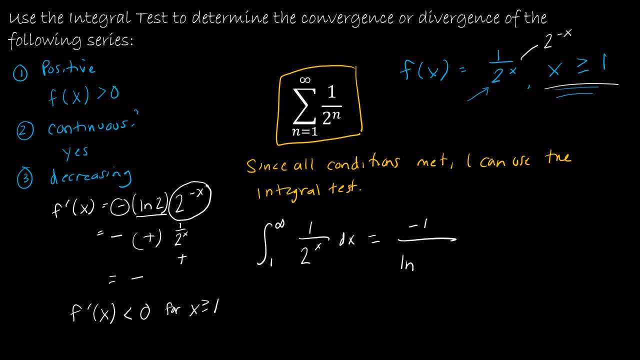 Now some more corrosive process, Reallyня? We see, theざsandra question is going to go all the number to羅 and the thing to be negative after 1 over the natural log of 2 times 2 to the x, from 1 to infinity, And again, if you don't remember, 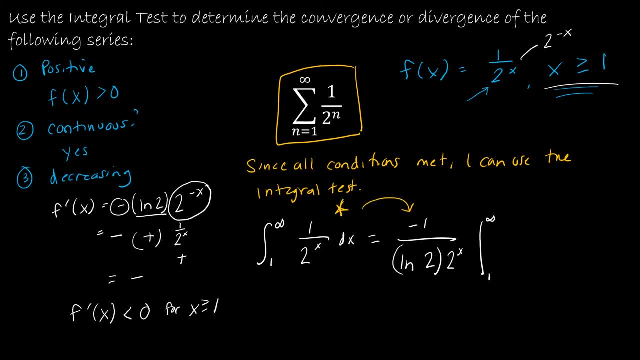 all of these rules, that turns 1 over 2 to the x into negative, 1 over the natural log of 2 times 2 to the x. that's okay. Just go back to your list that you had from Calculus 1 or Google to find a. 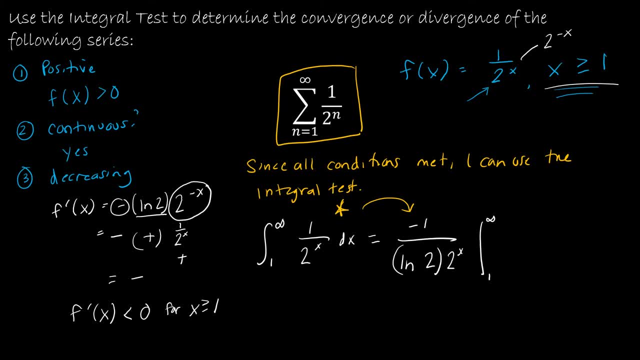 great informational sheet that has the derivatives and integrals that we use most often and you will find this pattern. So if you don't have it memorized, don't beat yourself up, that's just fine. So again, I'm going to think about this: If I'm plugging in infinity and 1,, I'm going to get. 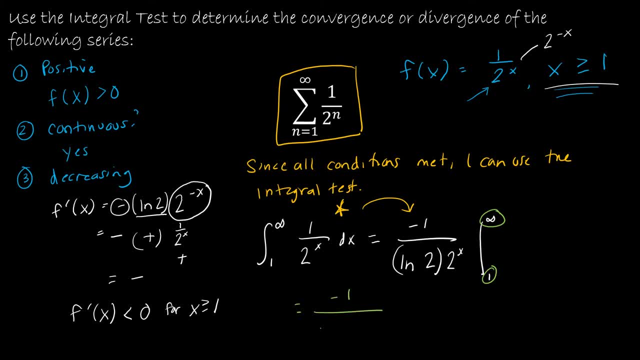 negative 1 times the natural log of 2, and then 2 essentially to the infinity. And then I'm going to subtract negative 1 times the natural log of 2 times 2 to the first. Well, 2 to the infinity is 0.. I'm sorry is a very large number, excuse me. 2 to the infinity. 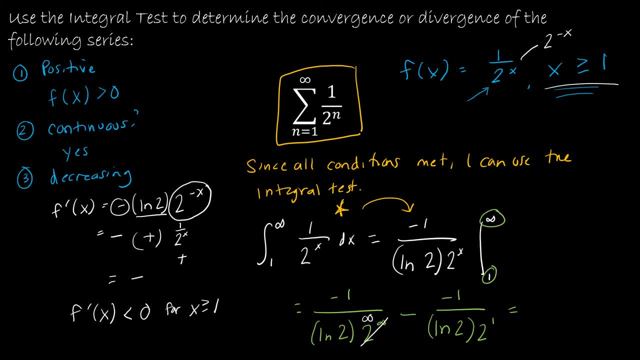 is a very large number and negative 1 divided by a very large number is 0. So this is essentially 0 minus negative, or 0 plus 1 over the natural log of 2 times 2.. And so this result is 1 over the natural log of 2, or 2 times the natural log of 2. is the way that. 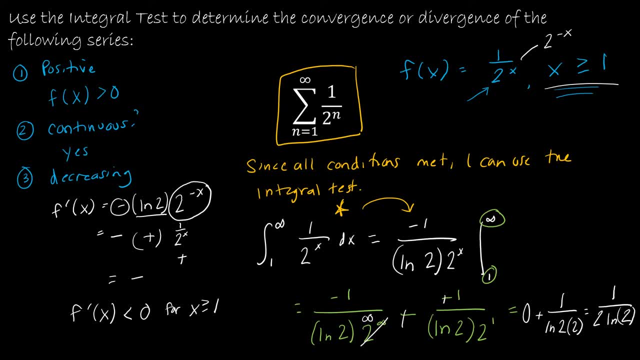 we would write that. Now. what does that mean? That means that because this integral converges to a value, that means that this series, so my series, the summation as n goes from 1 to infinity, of 1 over 2 to the n, converges by the integral test. 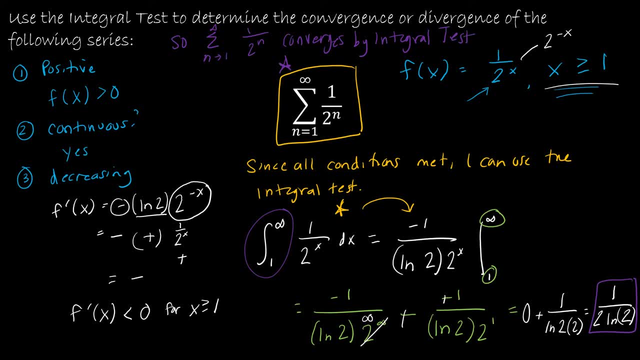 Now, what's very important to understand is that this summation does not converge to 1 over 2 times the natural log of 2.. That's not what this rule is saying. The integral test says: hey, I can help you determine if it converges or diverges. 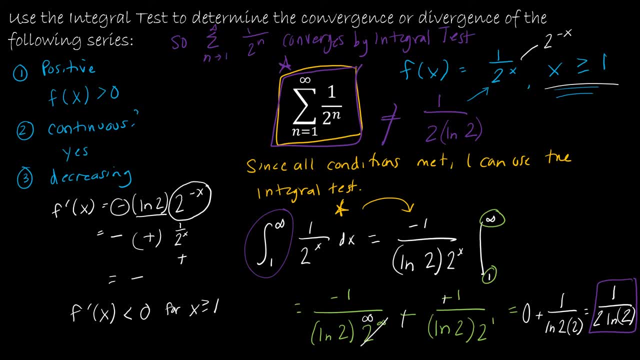 but I can't tell you what it's going to converge to. So we would have to have some other method to figure out what it converges to, Because this question doesn't ask for that. we're going to be done just by saying, yes, it converges by the integral test, but again, it does not converge. 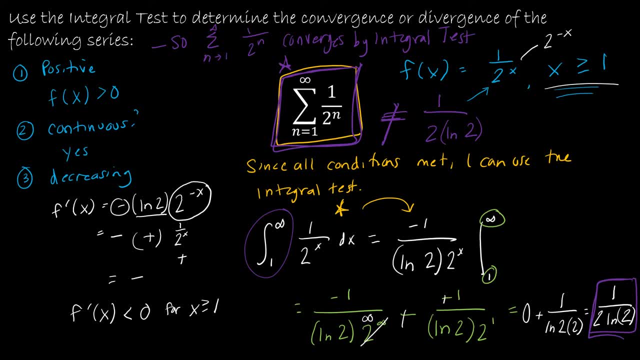 to the same thing that the integral results in Up. next we're going to take a look at the p-series. So let's take a look at the p-series.